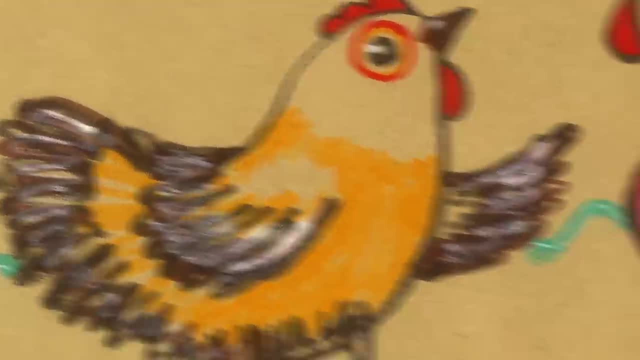 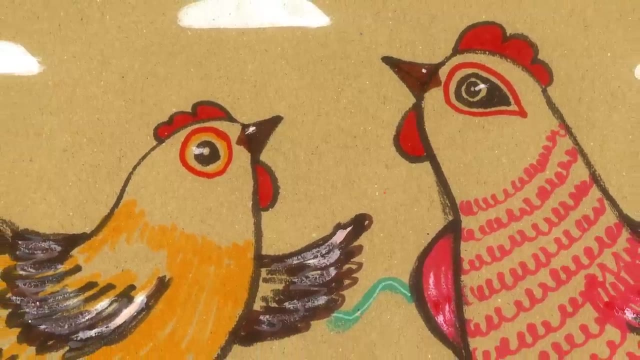 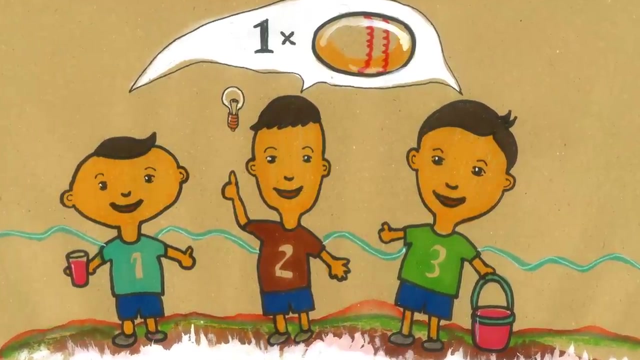 She decided then to look like Rosie, whose pink feathers looked so new and snazzy. Where did you get your feathers painted? Over there, where three boys waited, The first boy had a cup of pink ink. Give me an egg, I'll paint one feather pink. 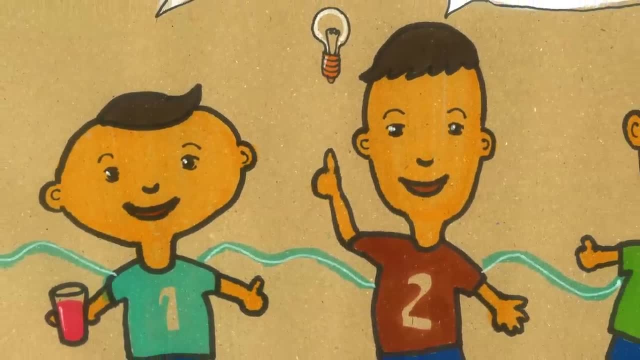 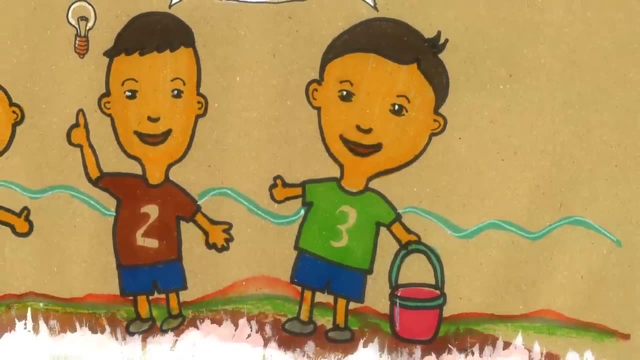 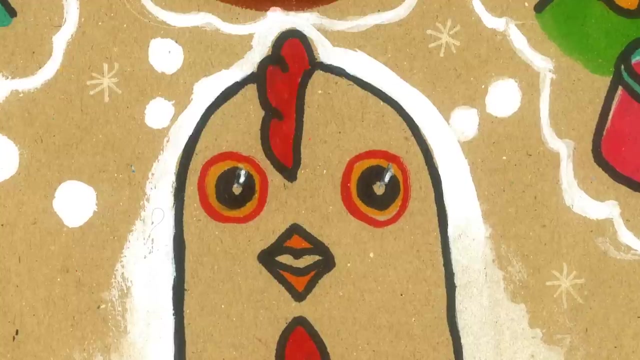 The second boy had nothing in hand. Give me an egg and I'll tell you my plan. The third boy had a pail of pink ink. Give me an egg, I'll paint ten feathers pink. Melissa stared at her three choices and in her head kind of heard these voices. 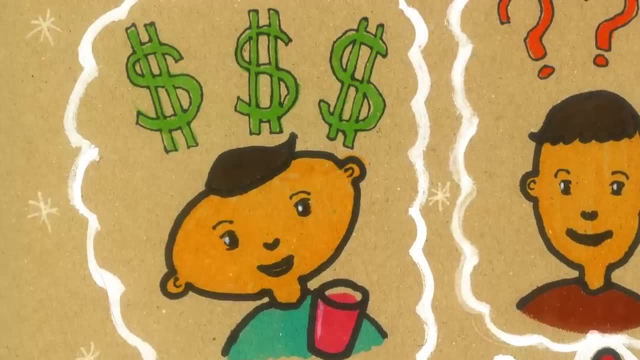 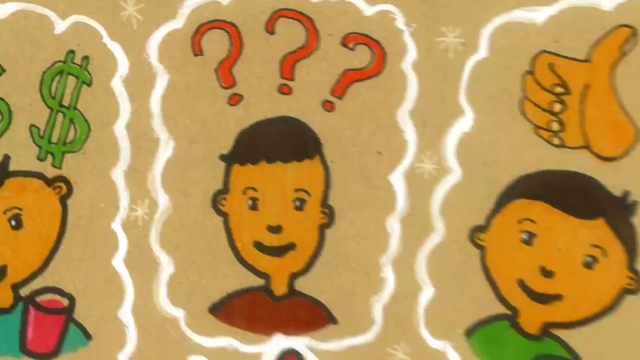 The first one's too expensive. You can't afford it. The second one's too cheap. Something fishy about it. The third one seems to be the best of the lot. That's what you should get. Give it all you've got. 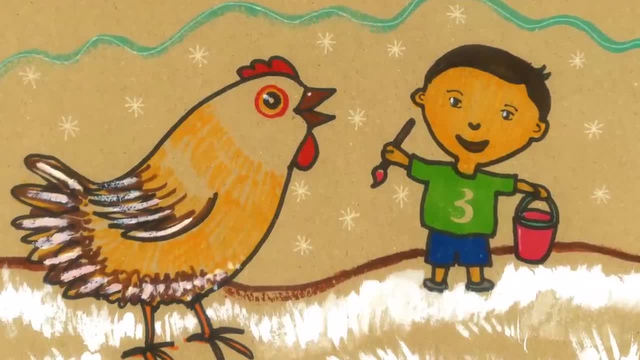 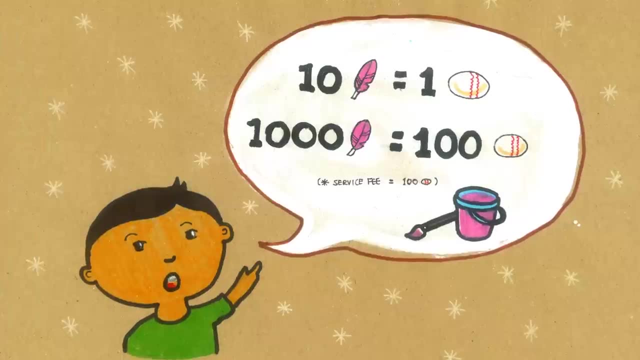 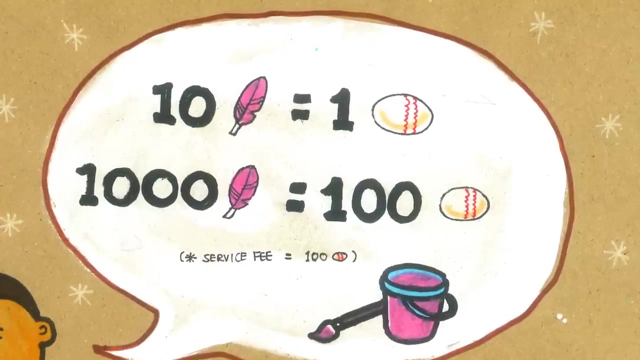 Oh boy, oh boy. Melissa told the third boy: I want to be pink, Give me your ink. You seem to have a thousand feathers, so that's a hundred eggs to paint your feathers. On top of that there's a service fee. 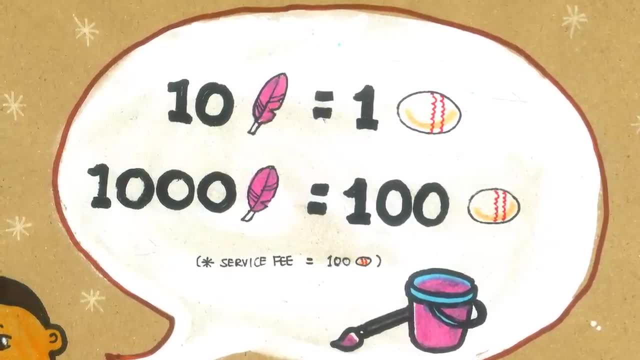 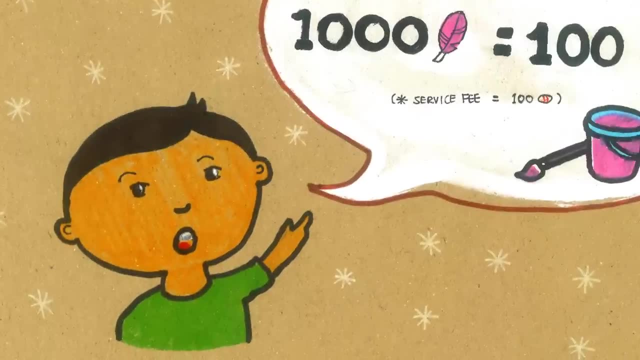 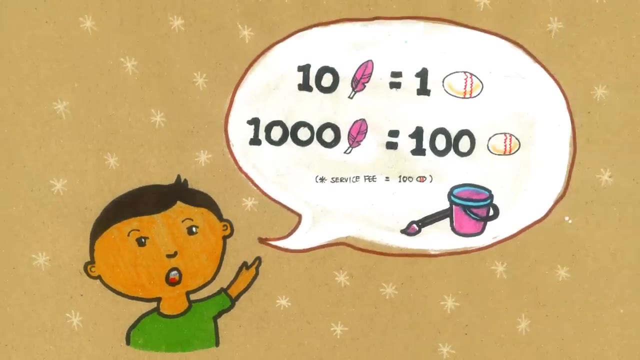 So a hundred more eggs for service from me. What said Melissa? horrified, You didn't say that. You mean you lied. It's not a lie, it's service charge. Ask them too, they'll all charge you. I don't have two hundred now, but I want pink feathers. so tell me how. 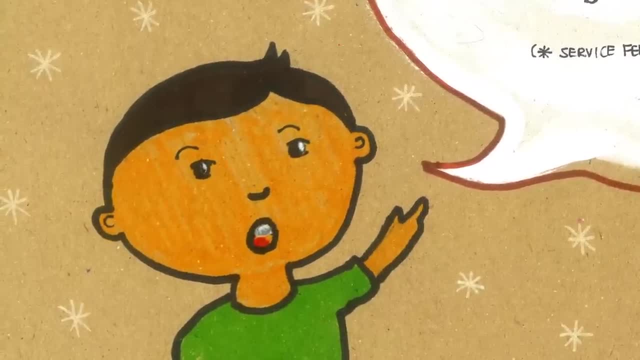 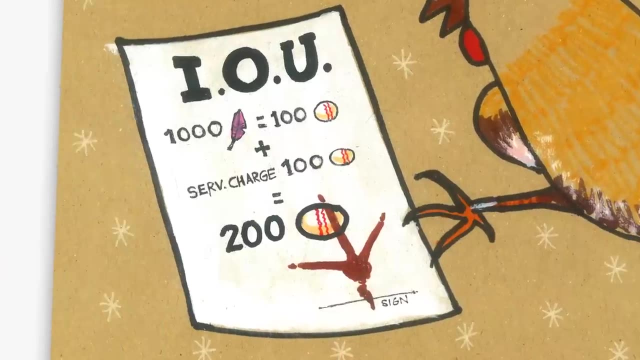 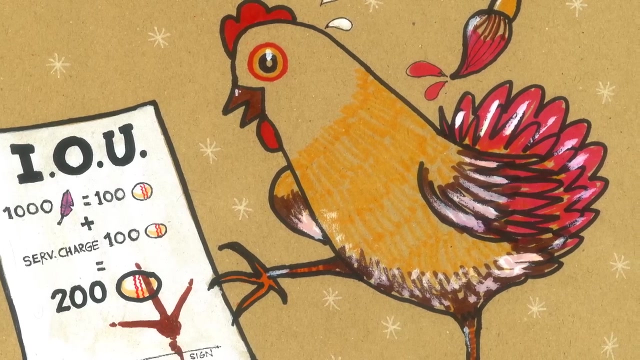 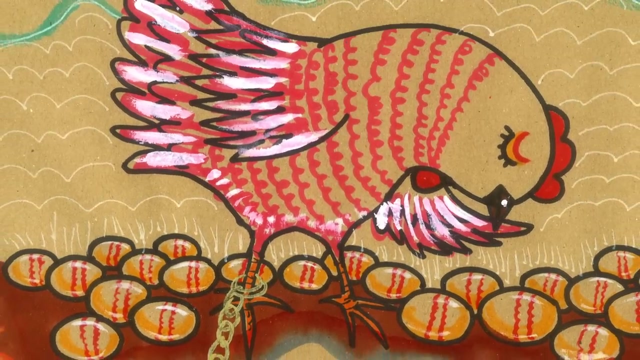 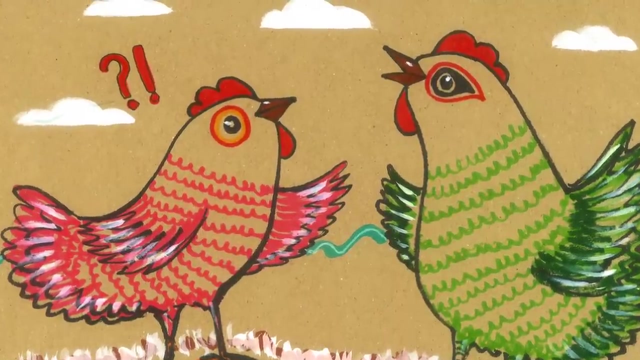 You can get a credit line and pay slowly over time. Melissa agreed and signed an ink and instantly got her feathers pink. But now, in debt, she laid eggs for the boy. For two hundred days she had no joy. The next time she saw Rosie again, Rosie's feathers were green.